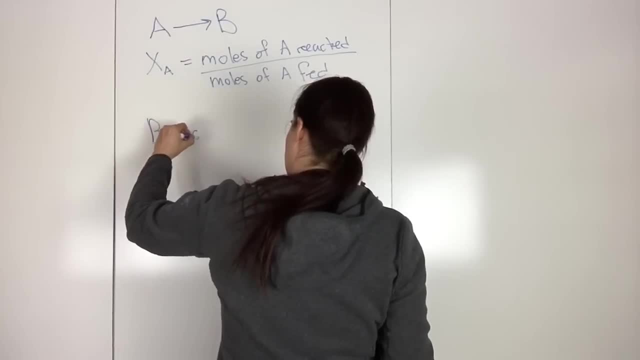 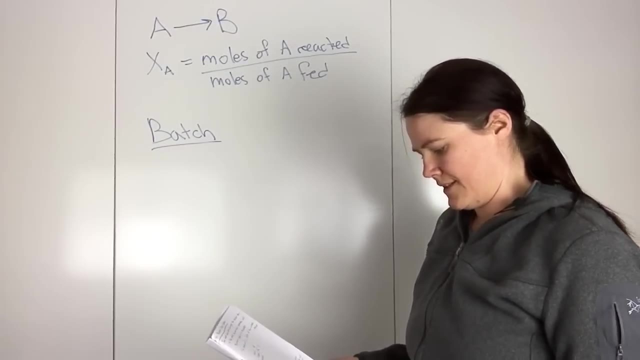 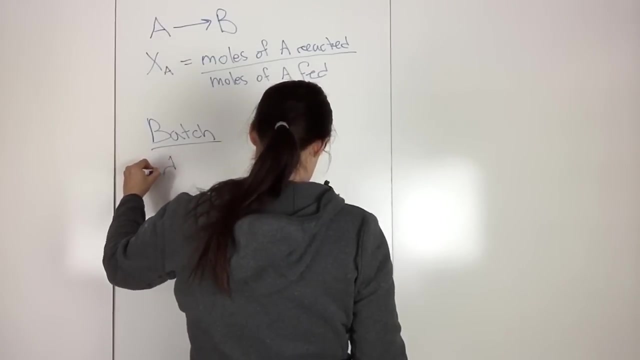 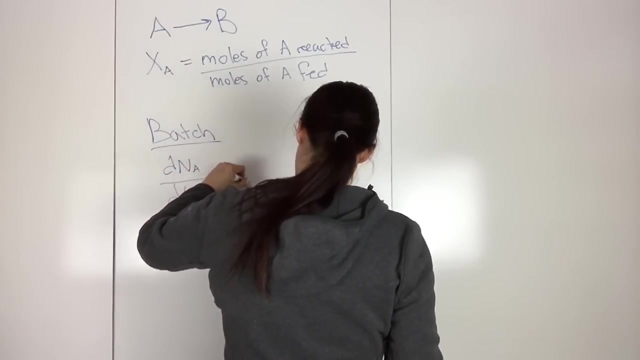 batch reactor, And we already know that the, that, the, the. the mole balance for a batch reactor looks something like this: So DNA over DT equals RAV. And if you want to know where this equation came from, it's in chapter one of Fogler's. 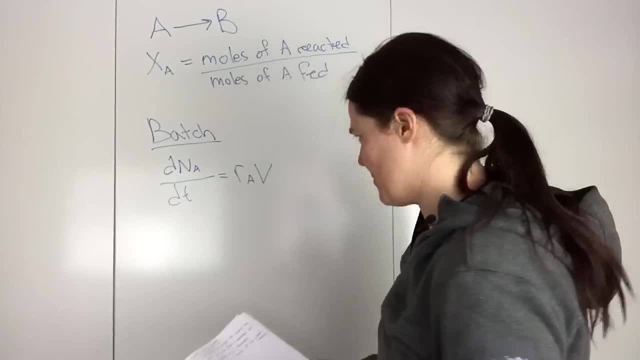 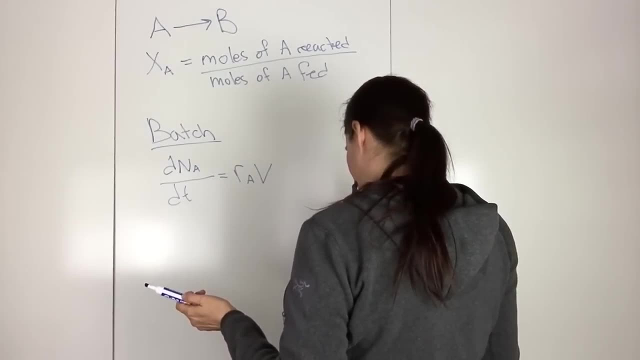 and I also derived it in a previous video. but it's just a mole balance And so what we want to do is write this equation in terms of this, in terms of conversion. So we need to relate this somehow. So, first of all, we know that NA, so this is the moles in the system. 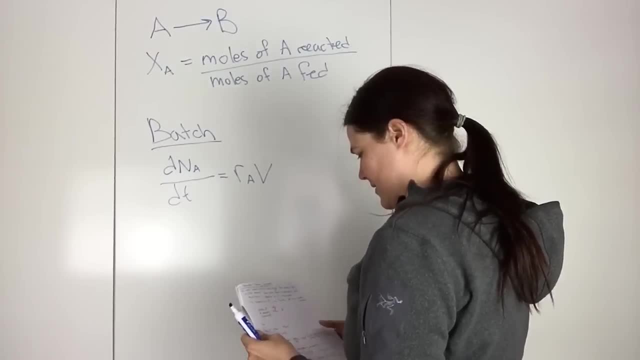 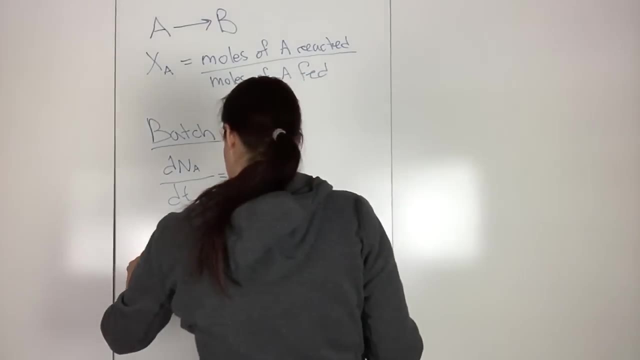 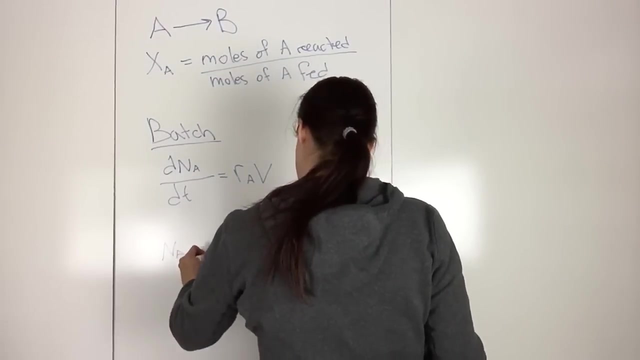 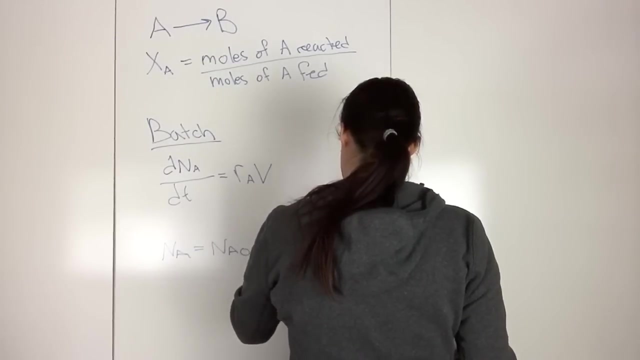 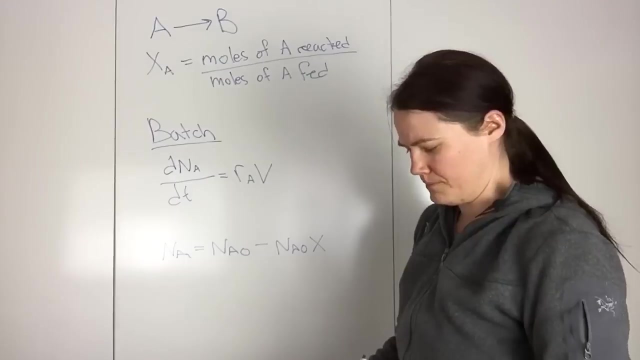 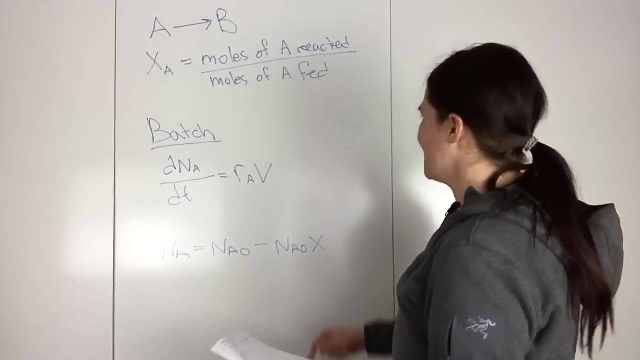 So we need to relate this somehow. So first of all we know that NA, so this is the moles in the system. So P-Q is equal to NA naught minus NA naught multiplied by the conversion. And you can see that that is the case from that equation. So basically, the conversion tells you. 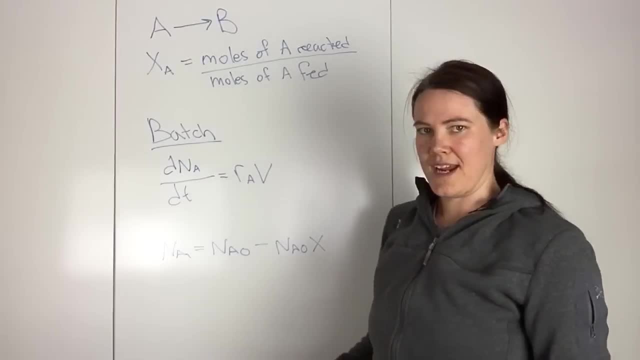 what percentage of A has reacted 양. so then, if you detect, if you detect this distribution, it's linked to, so this distribution, it's linked to nearly two A of four eighths. So there, there, there, there, So, there, there, there, there there's three A's, that is related to three. 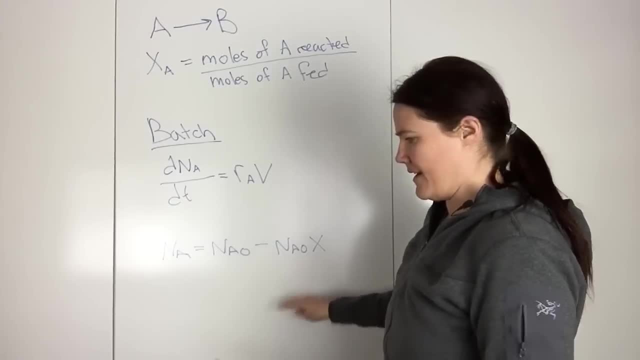 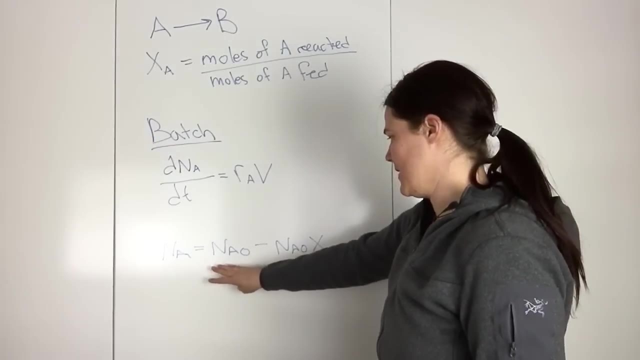 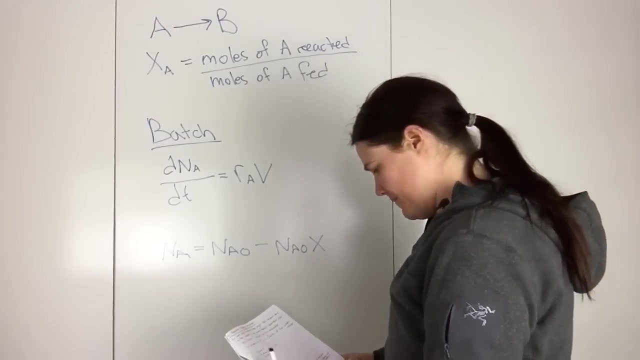 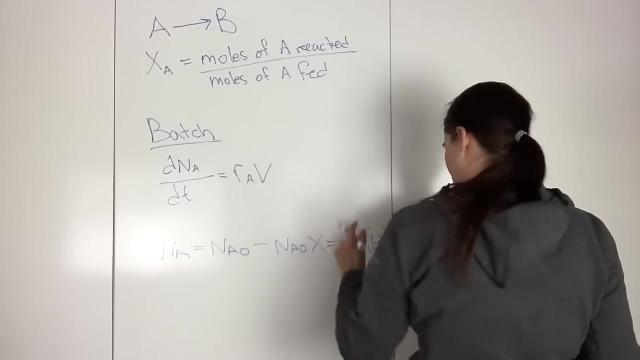 multiply that by this Na naught, then you know that this is the amount that has reacted, and so if you take the amount that you started with and subtract this, then that's what you have left. So this can be simplified to: Na naught 1 minus x. 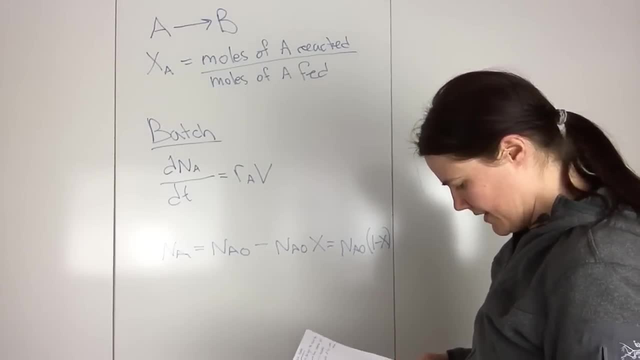 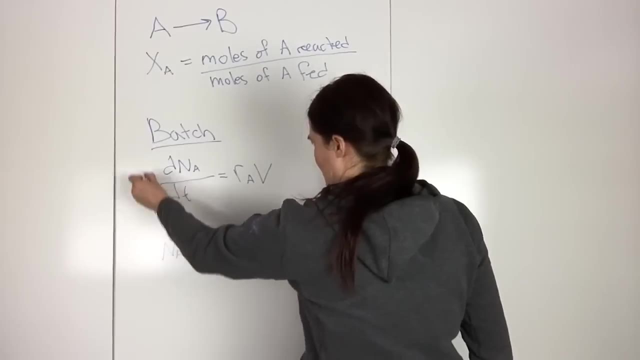 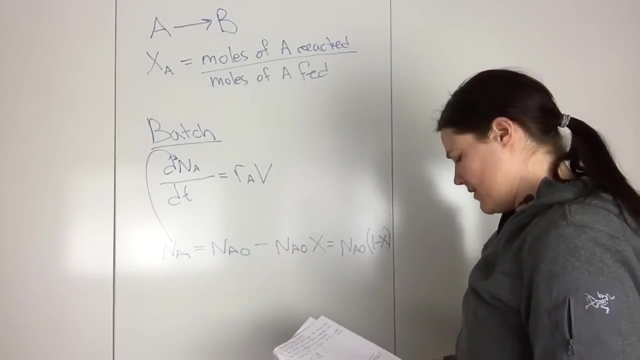 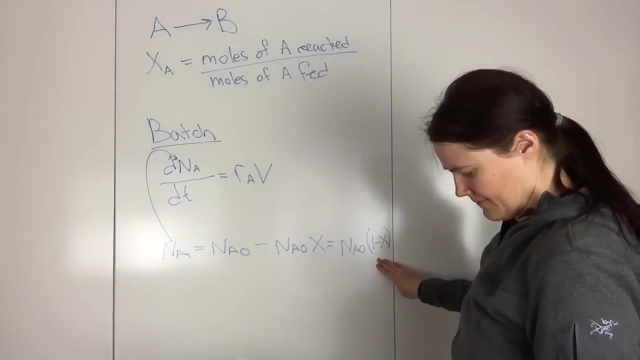 by pulling out the Na naught, And then we want to rewritebasically, we just want to plug that into there. So what we'll do is we'll write the mole balance in terms of conversion by differentiating this with respect to time, And we know that Na naught is constant. 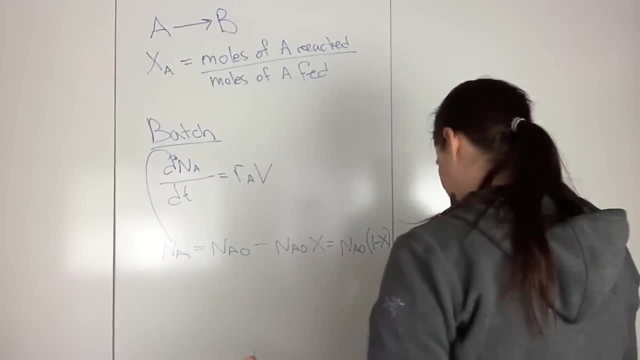 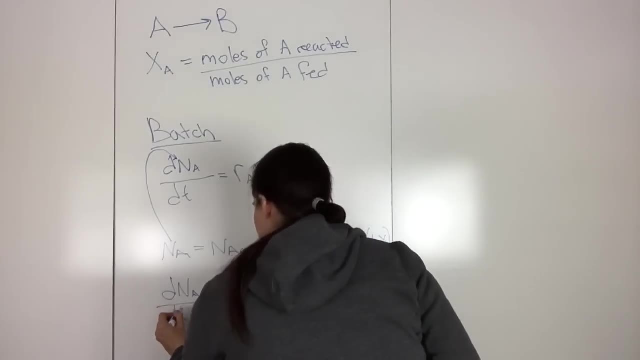 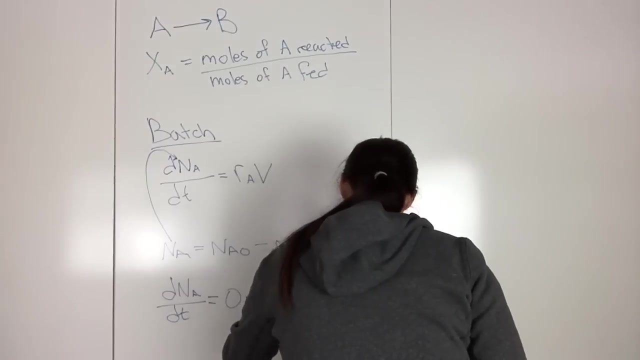 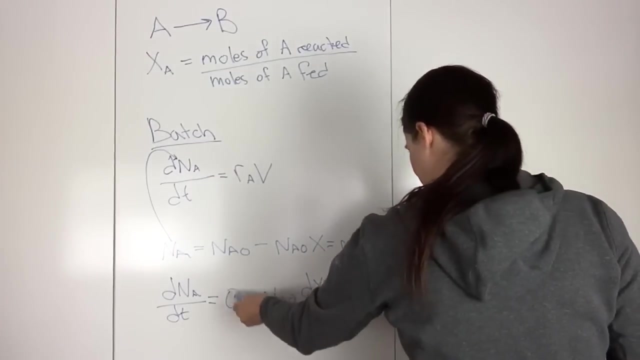 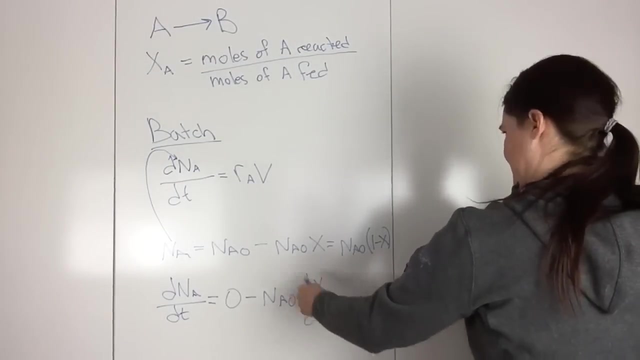 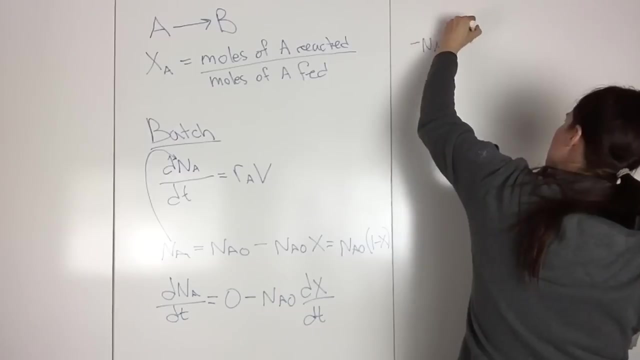 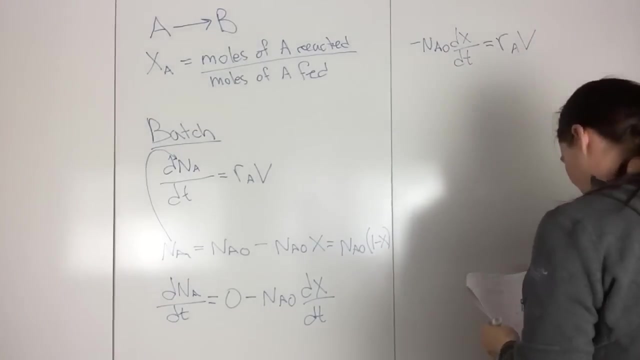 So we can rewrite this as dNa dT is equal to 0 minus Na0 dx dT, And so this is 0, because that's constant. So when we take the derivative it's just 0. And so then if we plug this back in, then we get minus Na0 dx dT is equal to Rav. 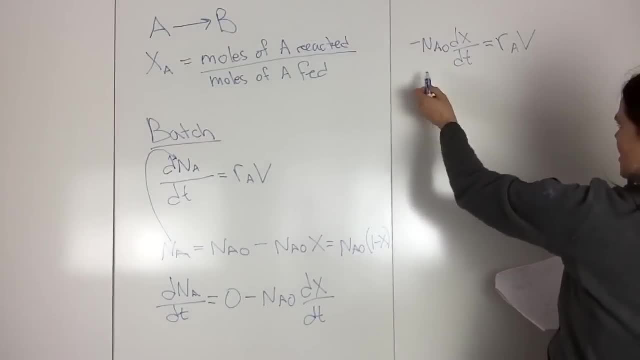 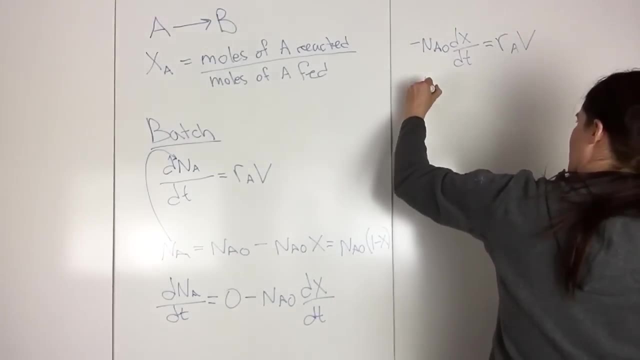 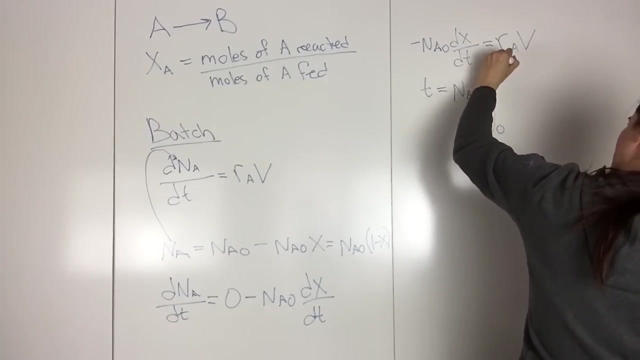 And then we can. so this is the differential form of the mole balance in terms of conversion for a batch reactor, And we can also write this in the integral form. So that would be: T equals Na0, 0 to x, dx minus Rav. 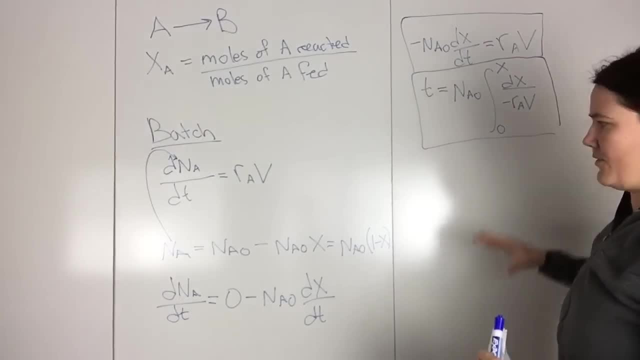 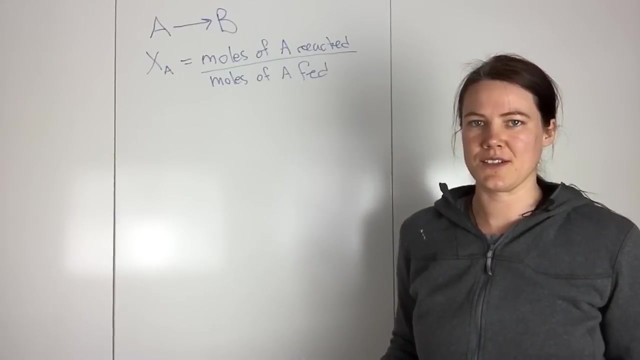 So this is the differential and integral form of the mole balance in terms of conversion for a batch reactor. Next, I want to write the. I want to rewrite the mole balances for the flow reactors in terms of conversion. So the first one I'm going to look at is the CSTR. 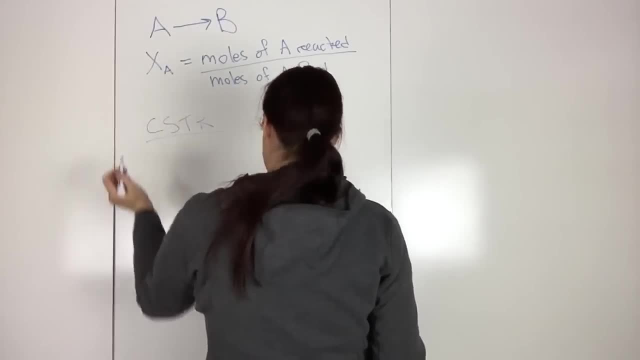 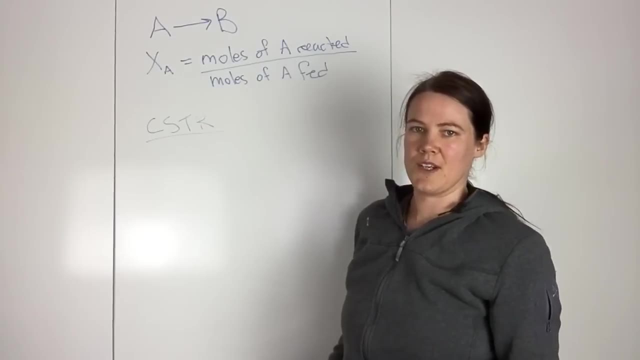 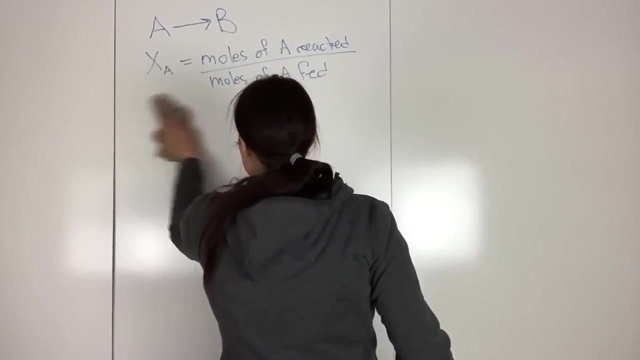 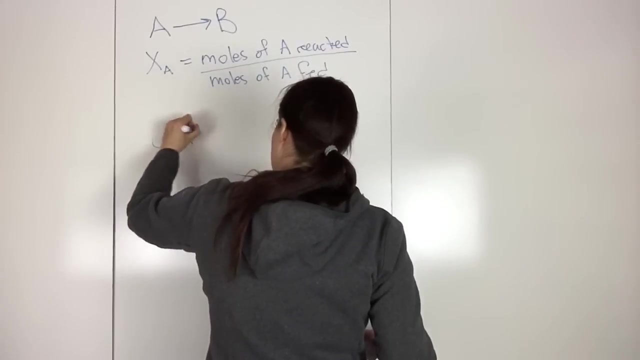 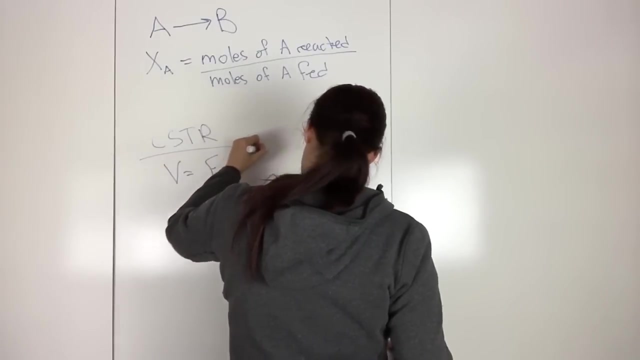 So this is for CSTR And if I write that, if I write down the design equation for that that was derived in chapter 1 and also in a previous video- that is V Alright. so V equals FA0 minus FA over the rate. 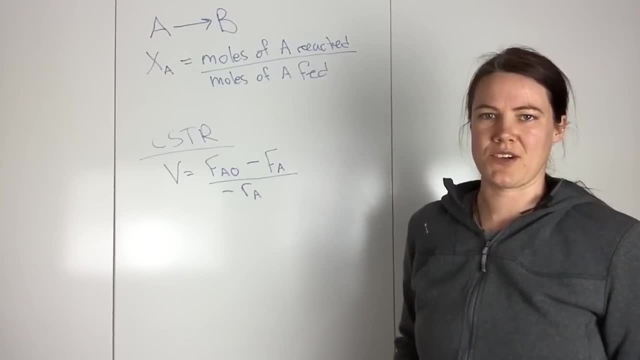 And so then we can kind of use the same method as with the batch reactor to, and so then we can kind of use the same method as with the batch reactor to, and so then we can kind of use the same method as with the batch reactor to. 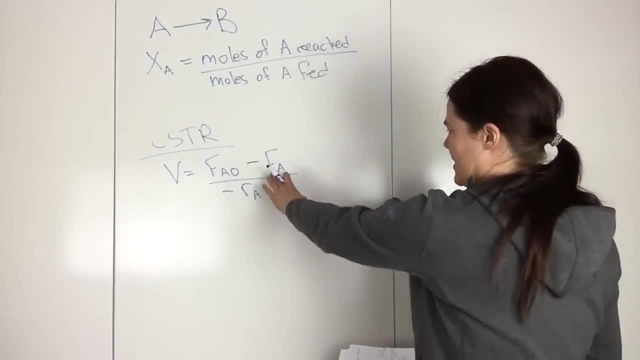 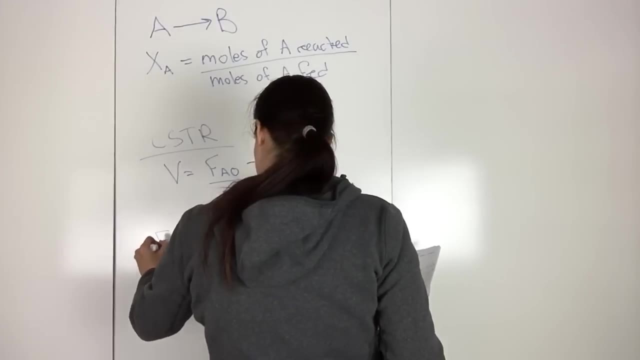 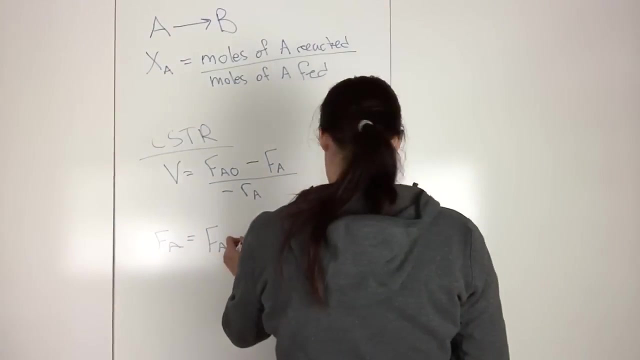 put this in terms of conversion. So we want to write an equation for FA in terms the molar flow rate, in terms of conversion. So we know that FA will be equal to FA0, which is what you have initially minus FA0 x. 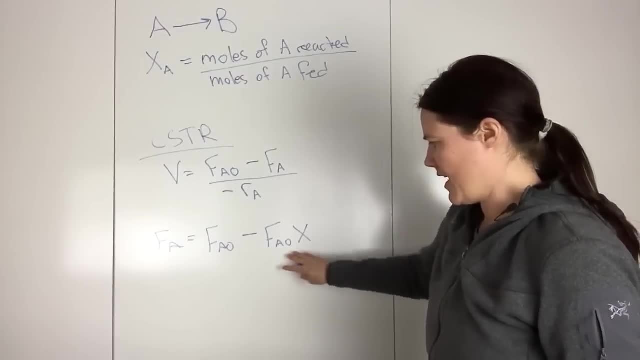 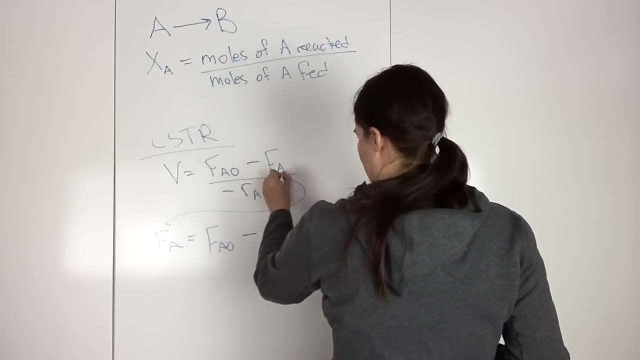 So what you have initially minus how much has been converted. So we know that FA will be equal to FA0, which is what you have initially minus FA0 x converted, And so that's what FA is. So then we can plug this in. 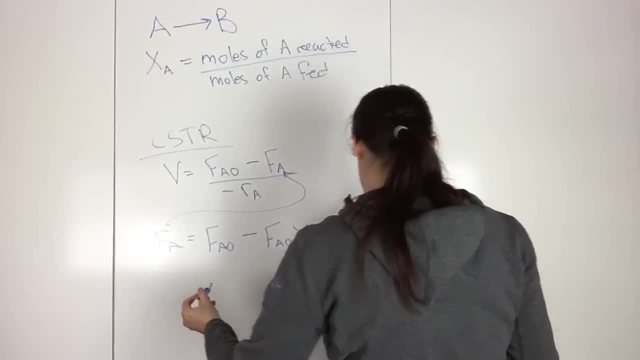 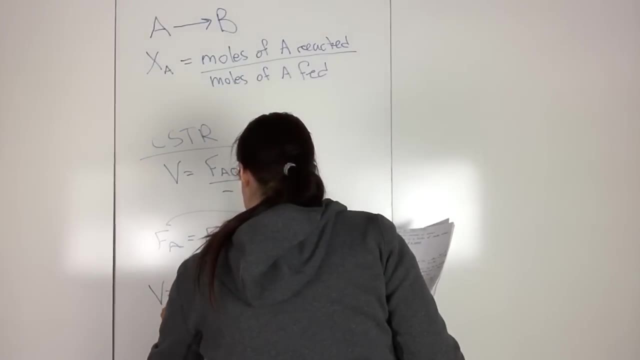 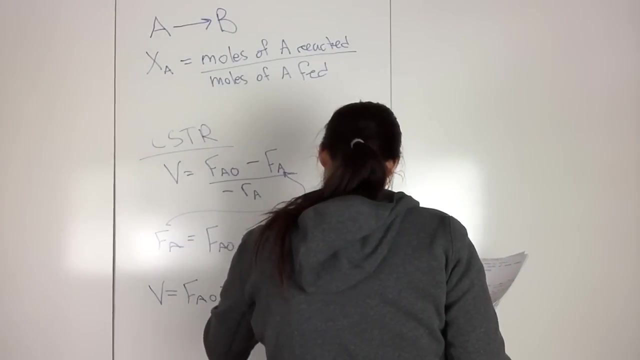 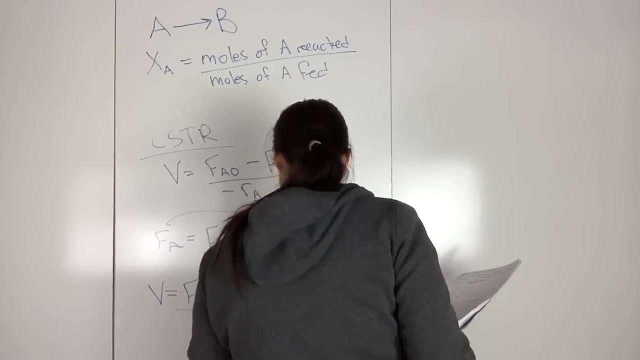 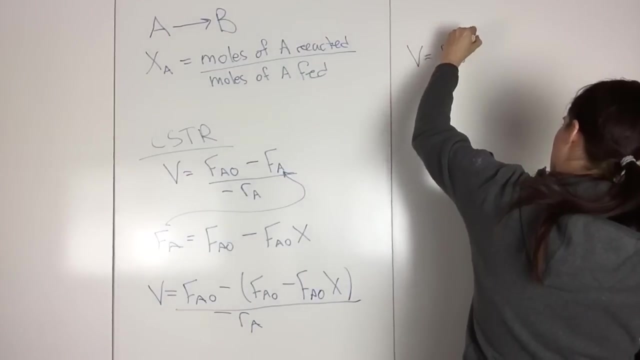 and get. so if you do that, you get V equal to FA0 minus FA0 minus FA 0 x minus FA 0 x minus FA 0 x minus R A, And so then this is equal to V, equals F A naught. 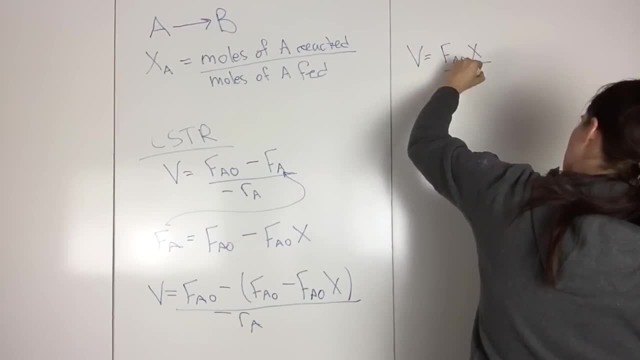 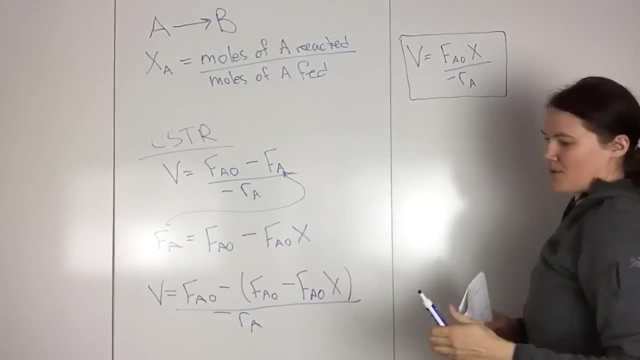 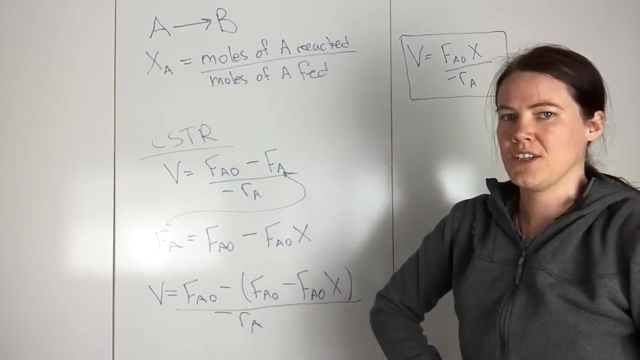 X over minus R, A over the rate. So then this is what's referred So, these equations that, when the mole balances are written in terms of conversion, they're often called the design equations for the various reactors. So this would be the design equation for: 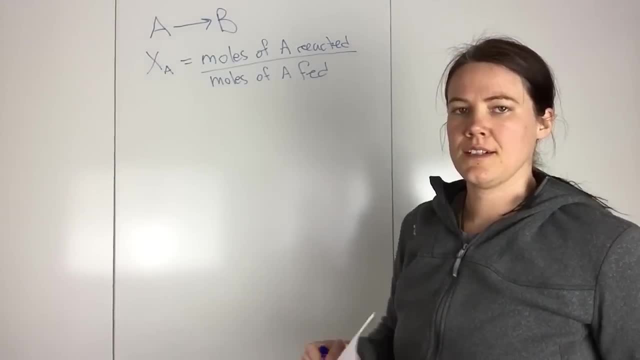 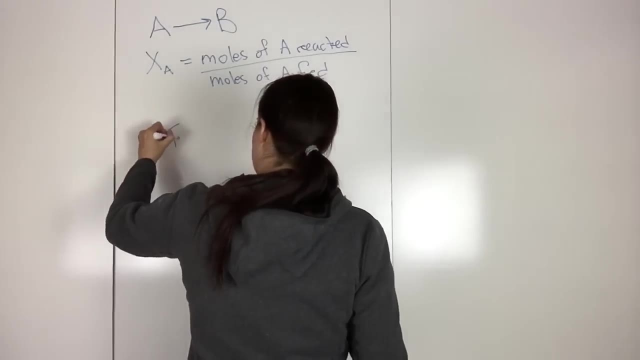 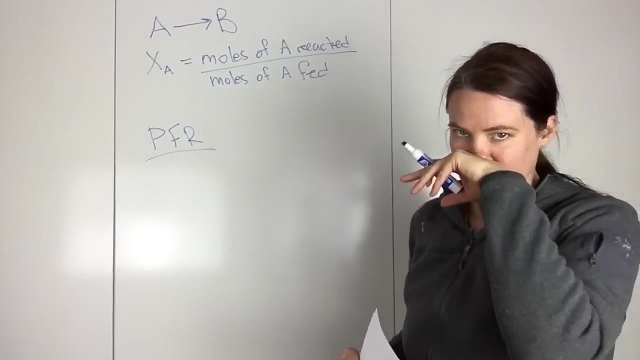 a CSTR. So I want to write the mole balance in terms of conversion or the design equation for a PFR, That's the plug flow reactor. So if I write down the mole balance that was derived in chapter 1, and also I did a video on this, then that 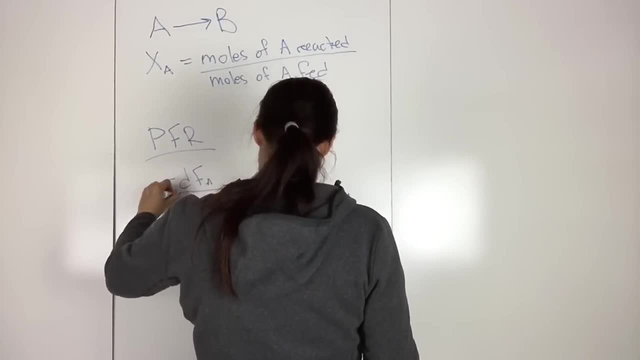 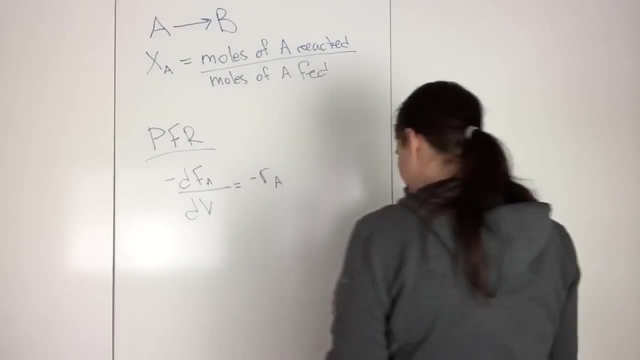 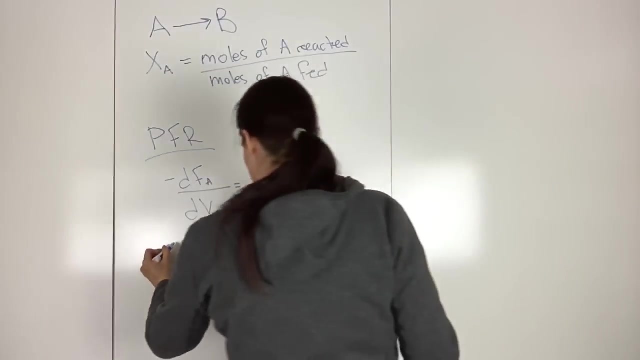 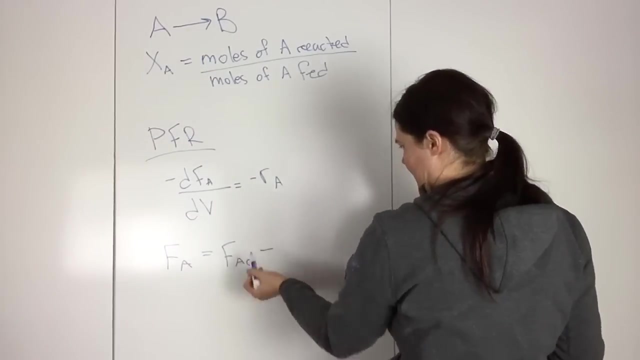 is minus DFA over DV, equals minus R A, And so then I can write down this molar flow rate again in terms of conversion. So that would be: F A is equal to F A- naught, what you started with. minus F A- naught. 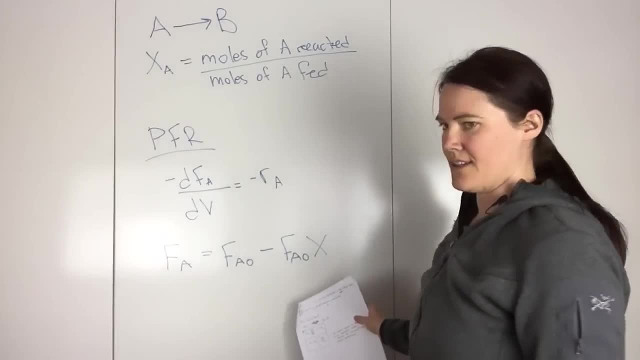 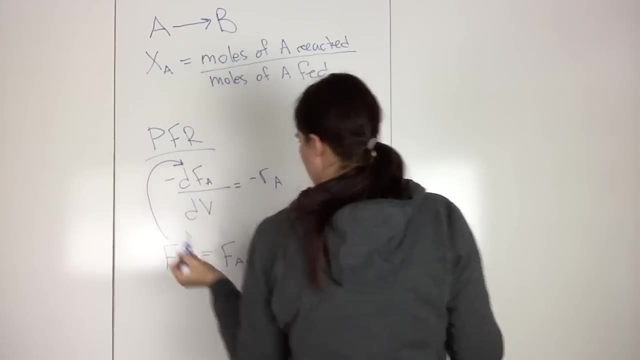 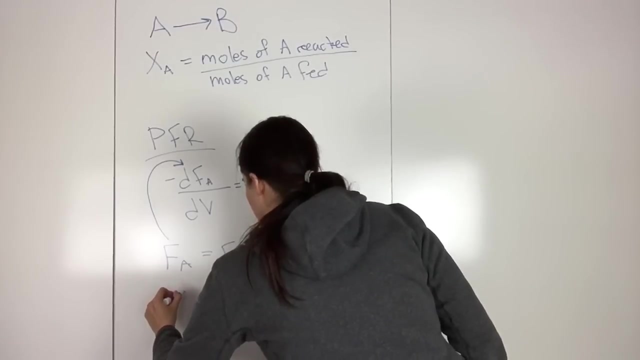 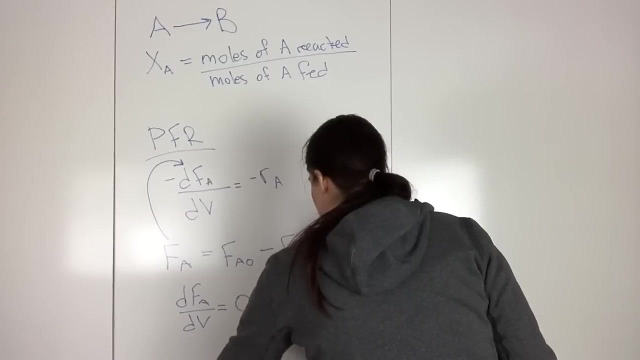 multiplied by conversion. So that gives you how much is been converted. And I want to plug this into here, And if we do that, we end up with let's see. so DFA DV is equal to zero minus F A naught DX DV. 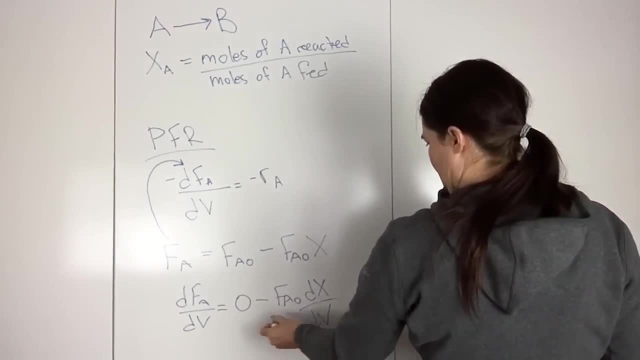 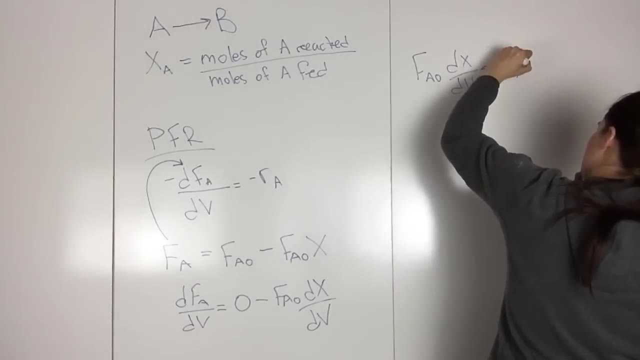 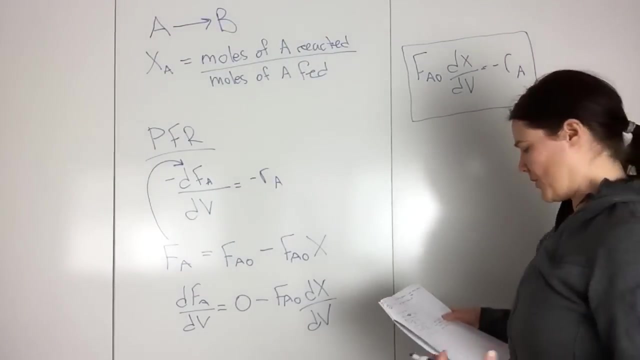 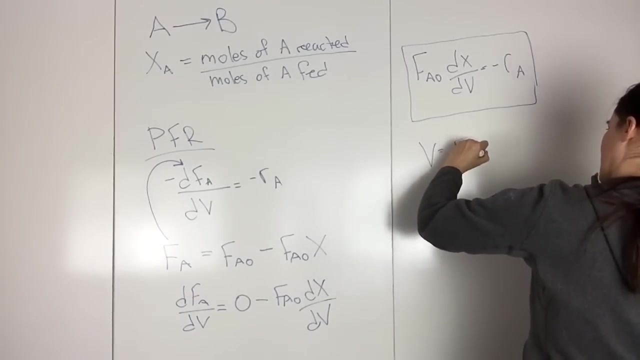 So then you just plug that in. so we have naught: DX DV is equal to minus R A. So then, this is the differential form of the design equation for a PFR, And this can also be written in integral form. So V equals F A naught. 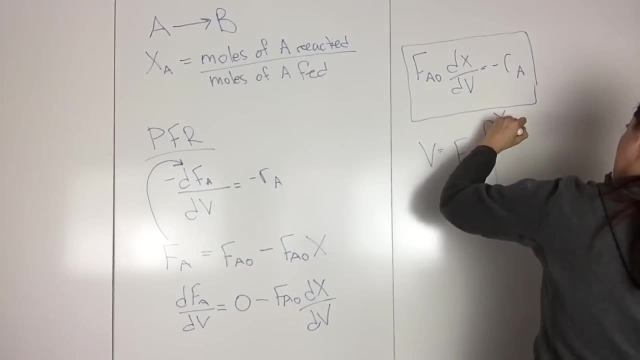 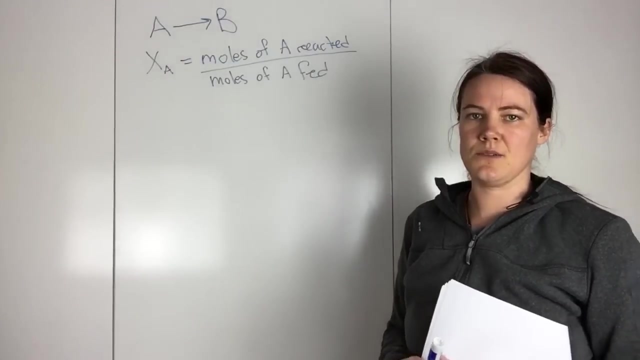 zero to X. So that's the differential form. So I can write down the PFR over minus R A. So these are the design equations in differential and integral form for a PFR. The last equation that I want to write, the design equation or the mole balance in terms of conversion for, is a packed bed reactor. 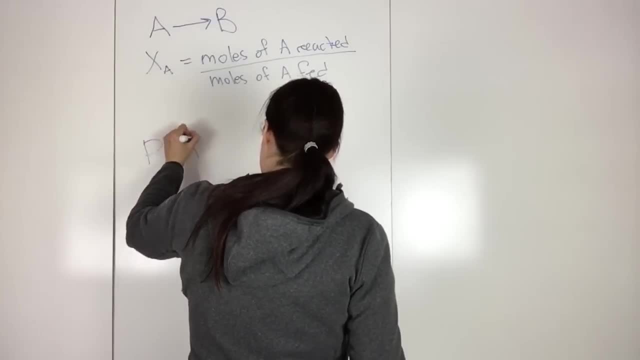 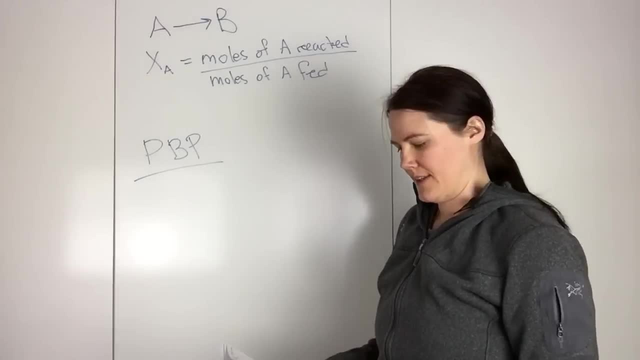 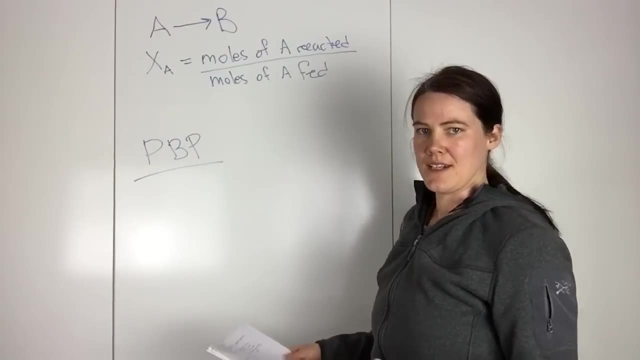 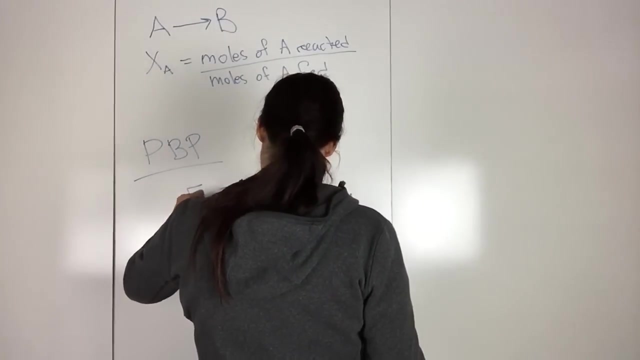 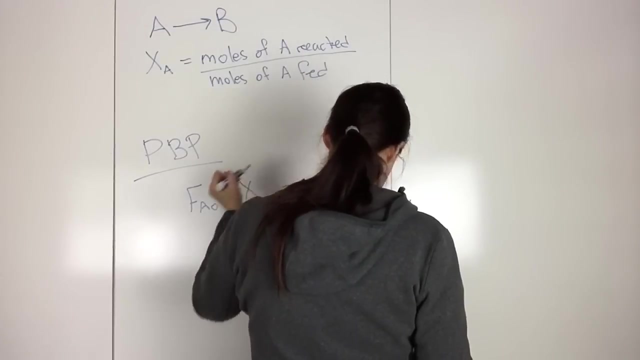 It's basically identical to the equation for a plug flow reactor, which is the one I just did. So I'm just going to write it down and the derivation is pretty much the same. So it is: F A naught DX. DW equals minus R A prime. 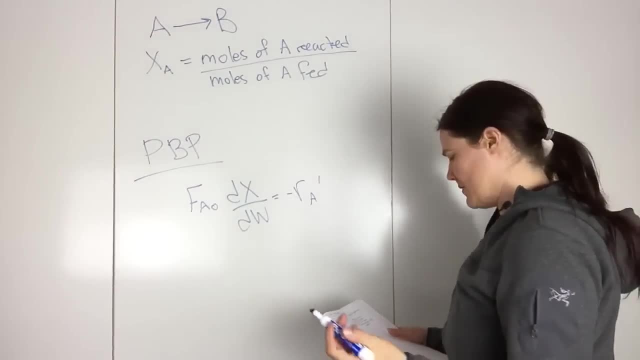 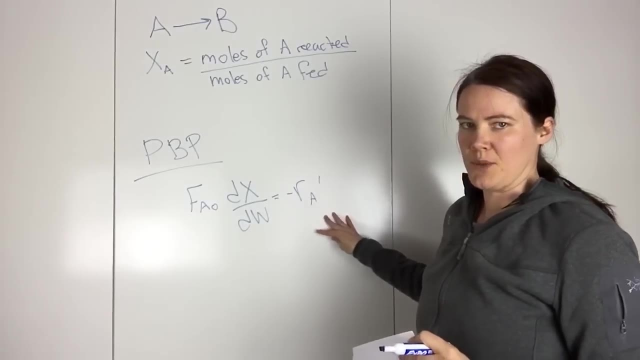 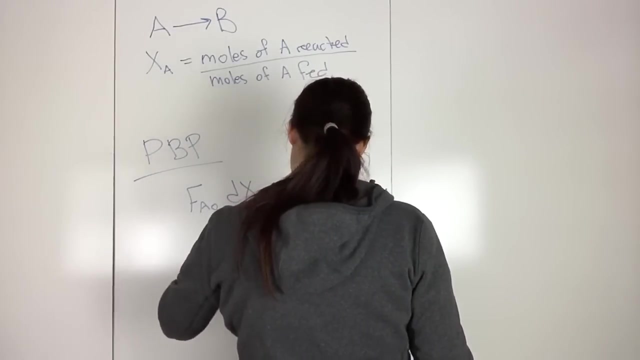 And then for this equation, if you so, for a packed bed reactor, you usually have a pressure drop, and so the differential form is normally used, but if you don't have a pressure drop, then you can use the integral form, which is this: 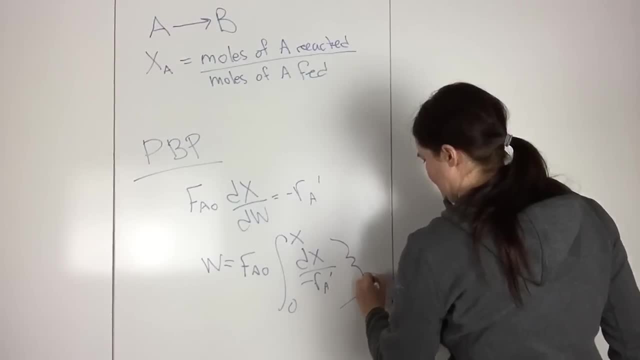 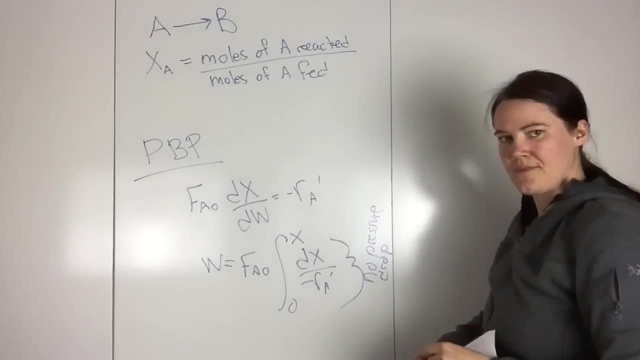 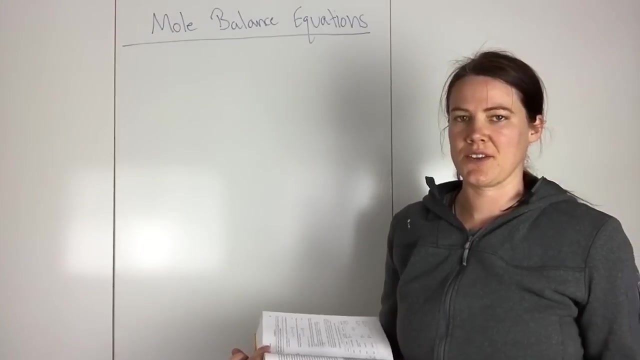 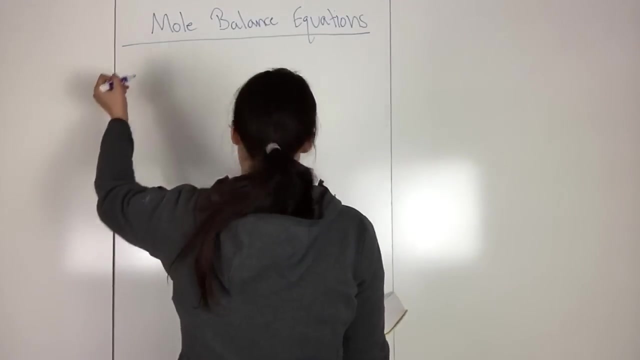 So remember that this form is no pressure drop. So I just wanted to quickly summarize all the equation derivations that I've gone through that are in chapter 1 and chapter 2.. So the first one is: well, so we did a batch reactor. 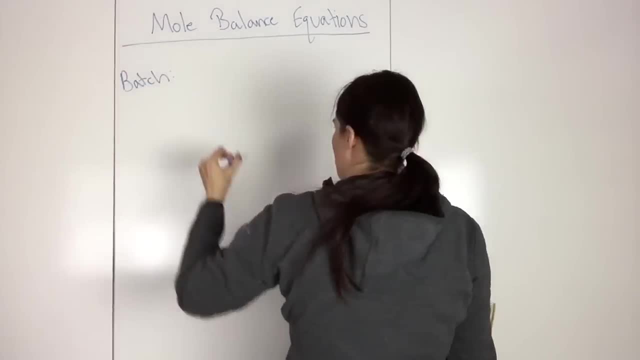 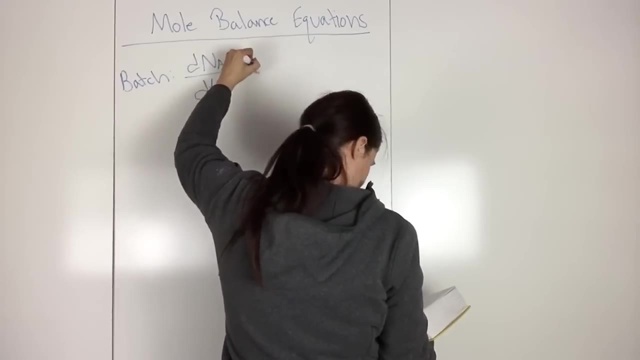 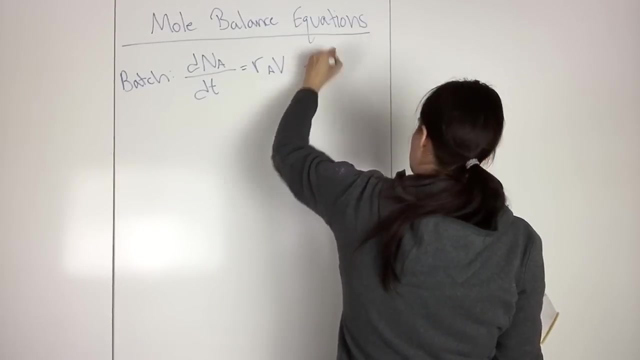 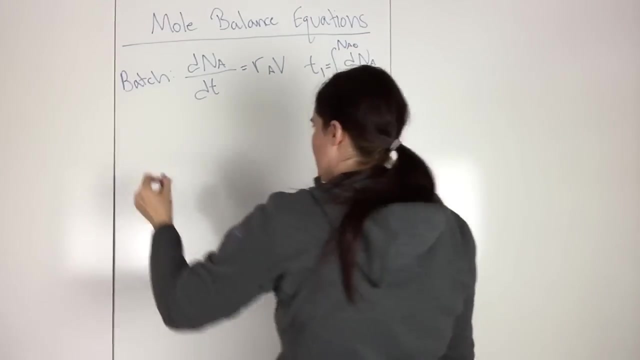 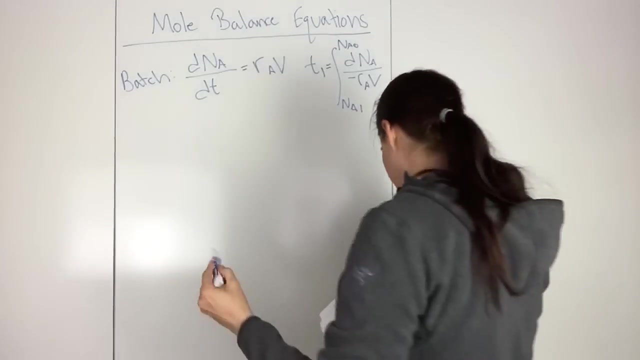 and the mole balance in differential form was this, And in integral form it was this: T1 equals Na1 to Na0, dNa minus Rab, And then for the N2 component, it's just the mole, And this also assumes that there's no 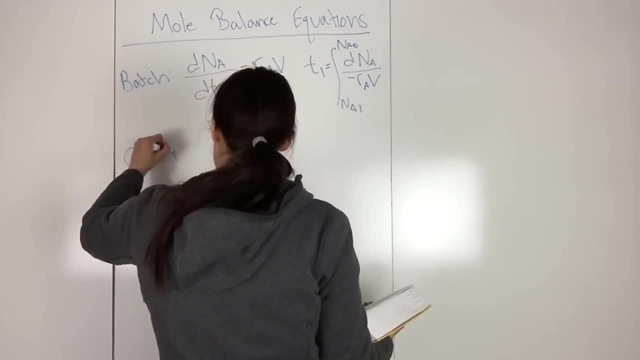 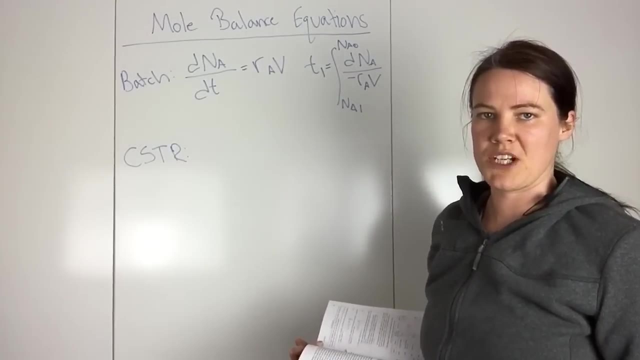 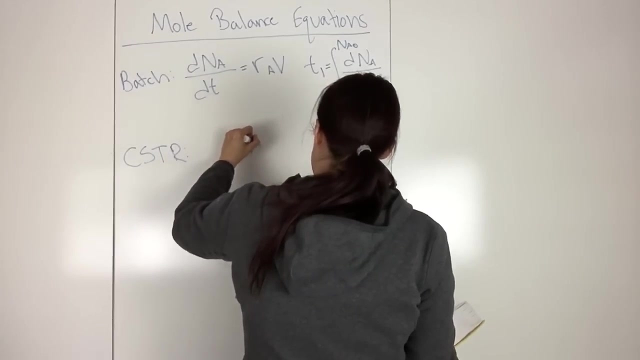 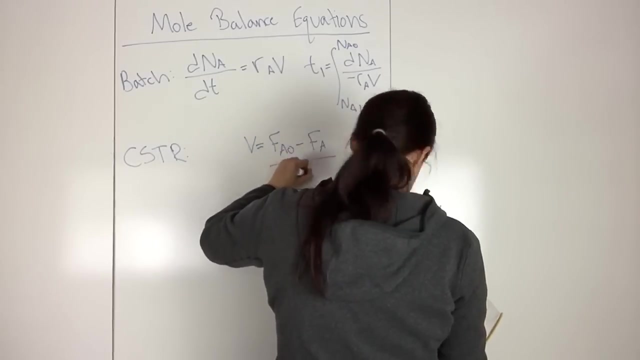 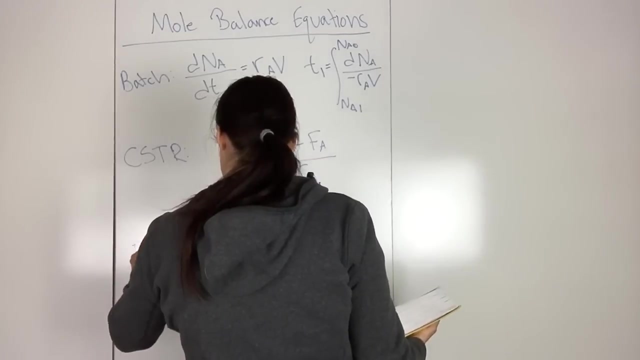 spatial variations in the reactor, and so for CSTR this. so for the CSTR, these equations assume also no spatial variations and they also assume that this is steady state. So this is just an algebraic equation. and then we had the PFR, and so the PFR assumes steady state for these equations. 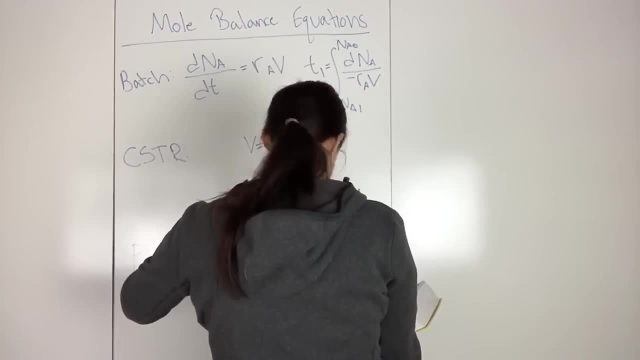 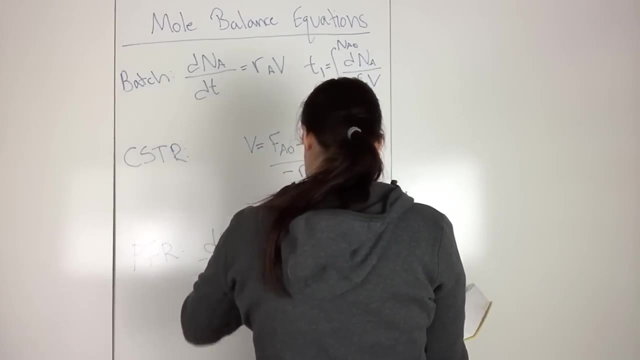 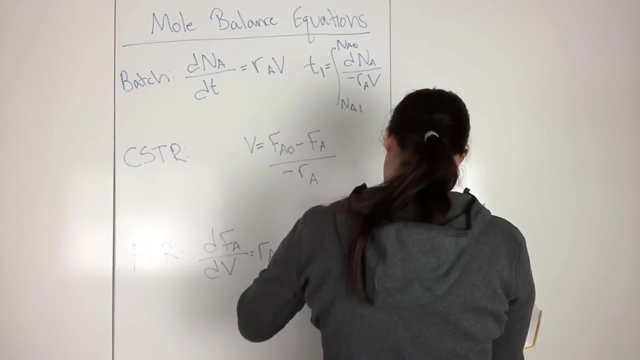 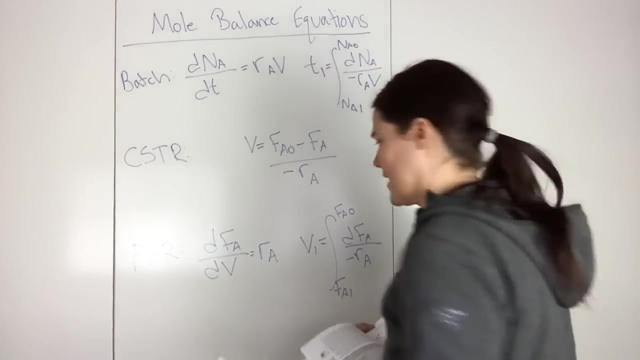 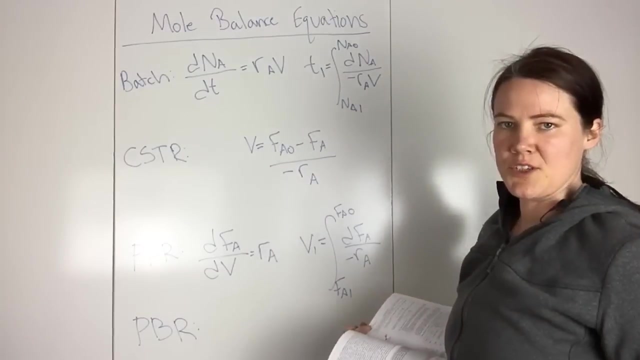 so the differential form was DFA. DV equals oops, equals the rate. and then in integral form the volume was equal to FA1. FA naught DFA over minus RA. and then the last one, the packed bed reactor, and this one also assumes steady state, so this was DFA. 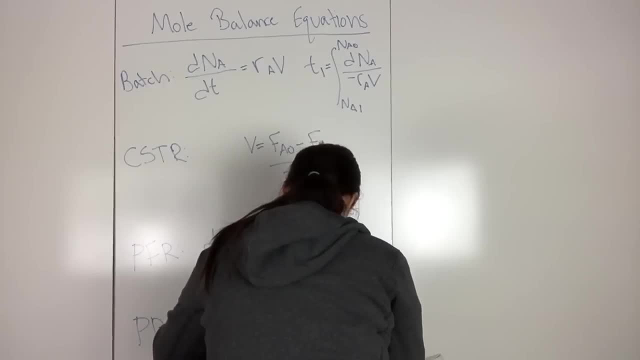 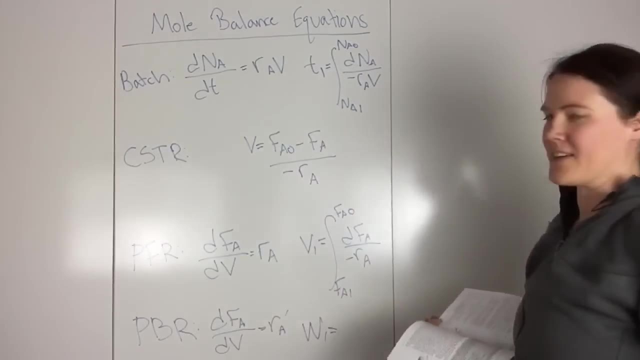 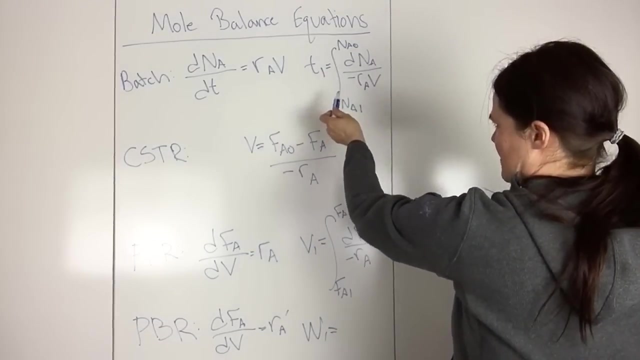 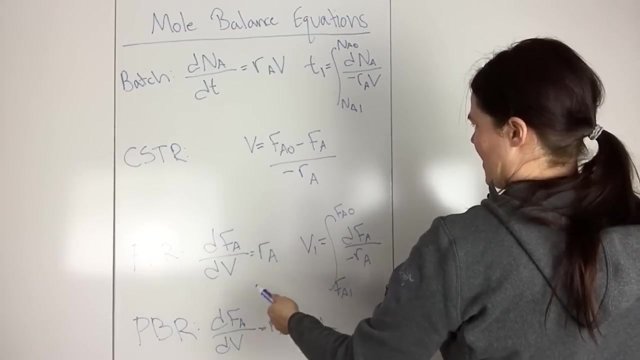 DV is equal to RA prime. and then the weight, because, remember, for the packed bed reactor you're interested in the weight as opposed to the volume. so for batch reactor, you're interested in the time spent, the time that whatever's reacting is spent in the reactor. for the flow reactors, the CSTR and the PFR, 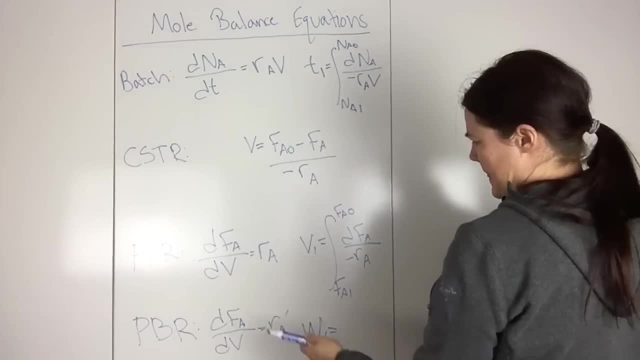 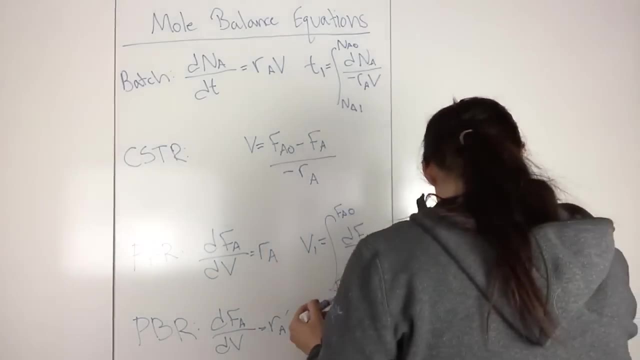 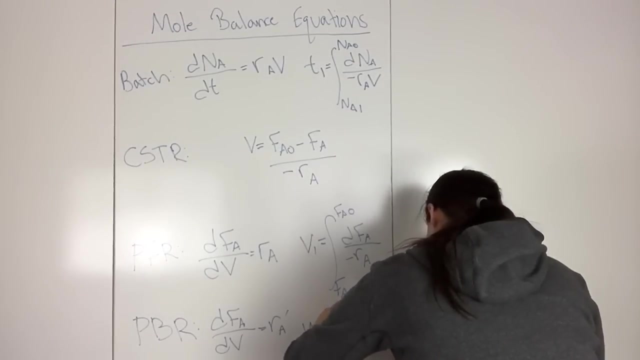 you're interested in the volume of the reactor. for the packed bed reactor, you're interested in the weight, because the reaction is based on the amount of catalyst you have. so this is the weight of the catalyst. so the weight is FA1, FA naught to DFA over R A prime. so then, skipping to the equations that we 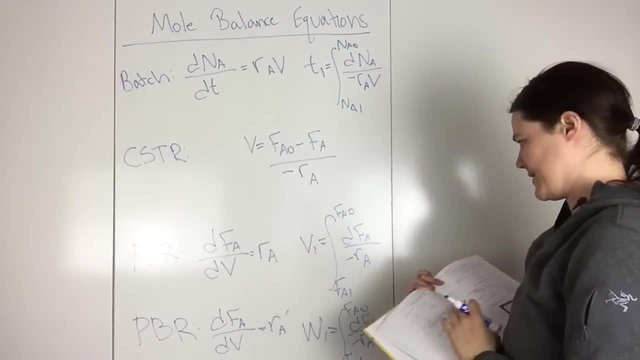 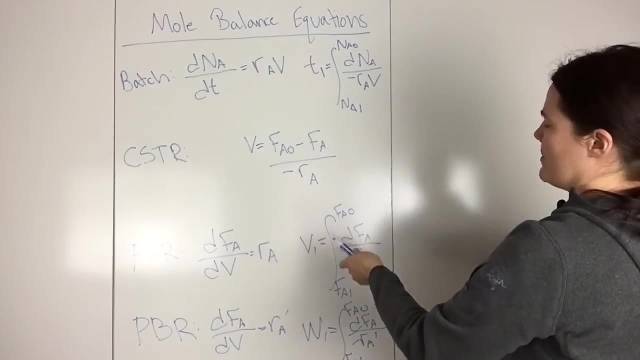 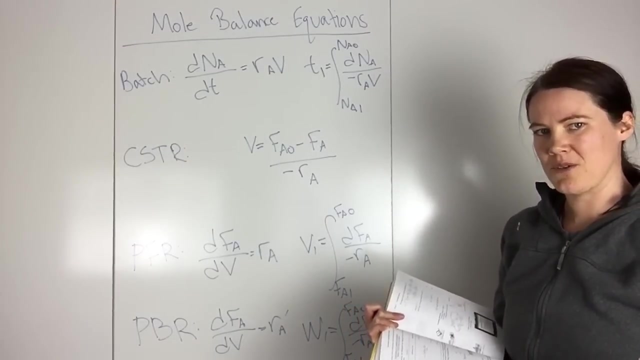 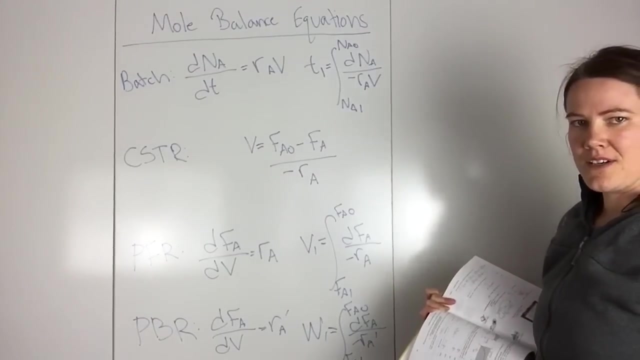 just derived. so these are the general mole balances, and so then we, in this video, we- we didn't read- derive these, but we converted them so that they were a function of conversion. so it's basically the same equation, but it's just a function of conversion, and so it's convenient if you're, if you have a 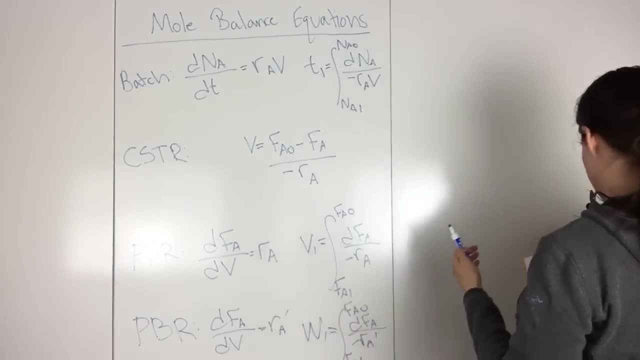 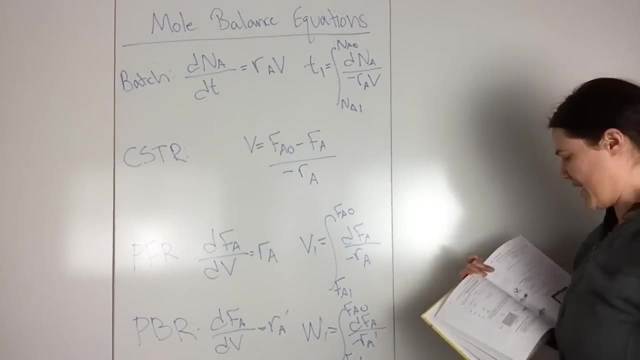 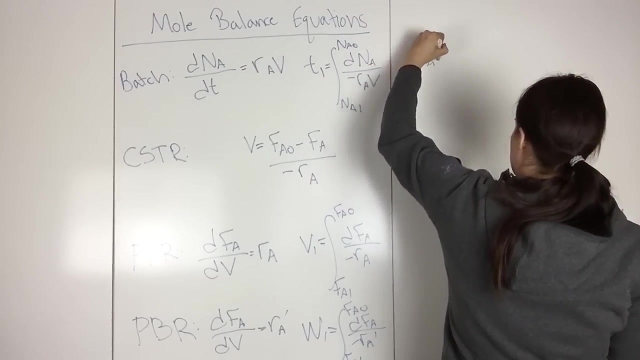 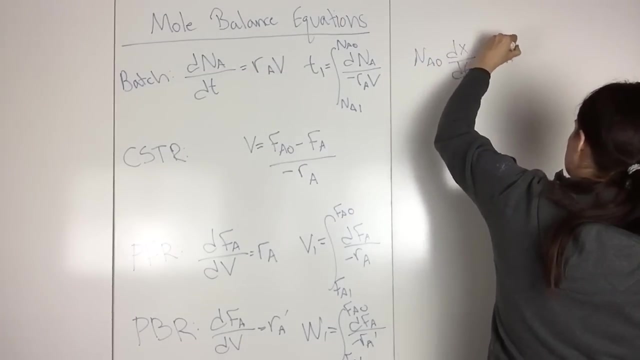 conversion, or if you're looking for a certain conversion, and so- and these equations are a function of conversion- are often called the design equations for these reactors. so, for the batch, the differential form of this equation was: NA, naught, DX, DT equals minus RAV and the differential form was: 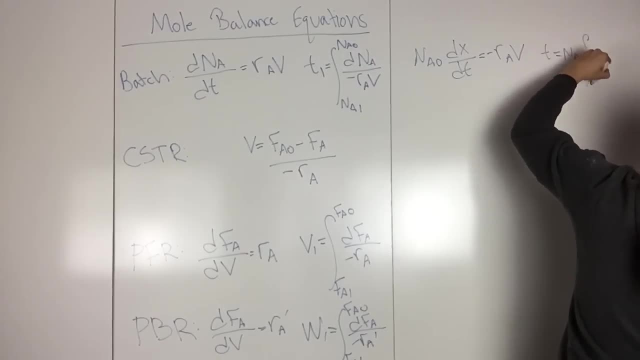 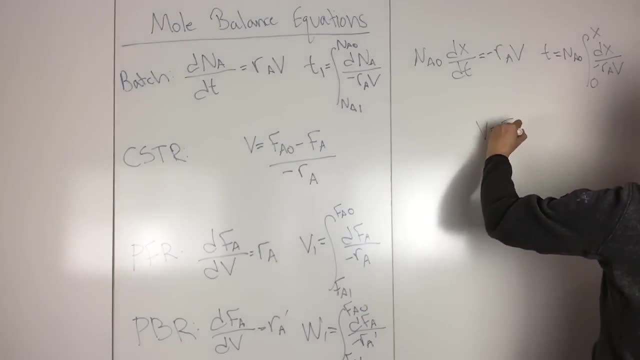 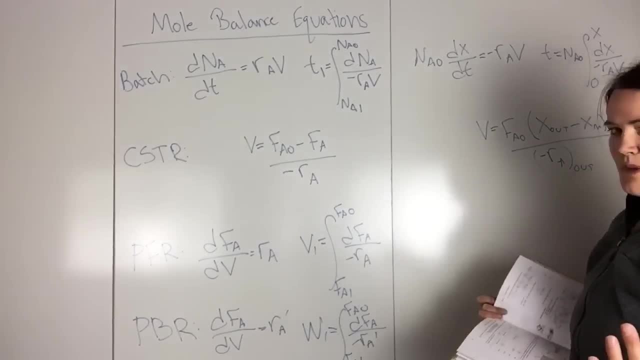 one reactor, but with these flow reactors you can have, you can have a bunch of them you can have. you can have a bunch of them you can have, you can have a bunch of them in series, and so your starting in series, and so your starting in series, and so your starting conversion might not be zero. so if you 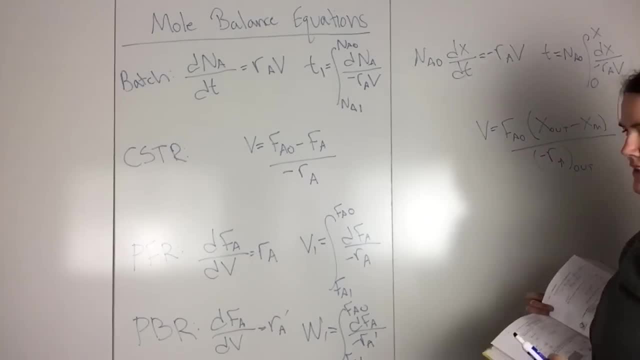 conversion might not be zero. so if you, conversion might not be zero. so if you just have one reactor, this X in is zero. just have one reactor, this X in is zero. just have one reactor, this X in is zero. so then you'll get the equation that I 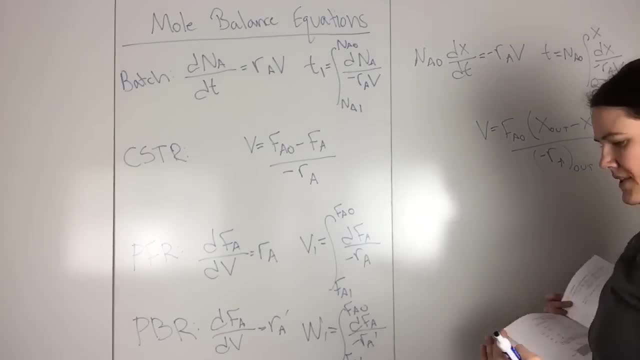 so then you'll get the equation that I, so then you'll get the equation that I derived earlier. but if you have a series derived earlier, but if you have a series derived earlier, but if you have a series of reactors, so you have one in front of. 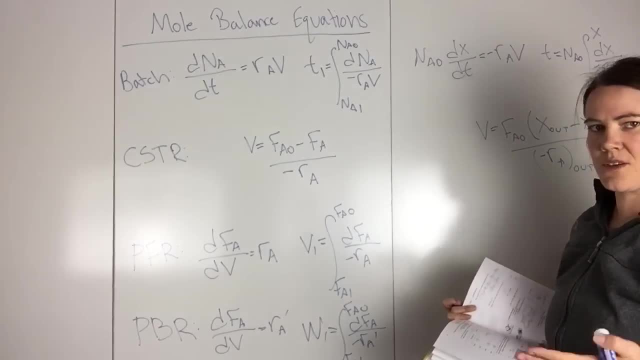 of reactors, so you have one in front of of reactors, so you have one in front of this one, then your conversion might be: something coming in, so then your X in something coming in, so then your X in something coming in, so then your X in would be: whatever the conversion is that. 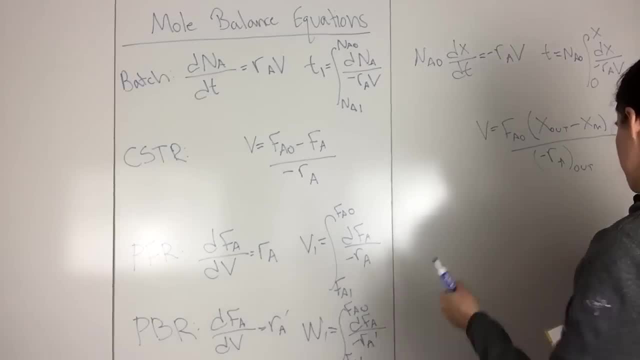 would be. whatever the conversion is, that would be. whatever the conversion is, that came out of the reactor in front of it, came out of the reactor in front of it, came out of the reactor in front of it. and you'll see that with these other two and you'll see that with these other two. 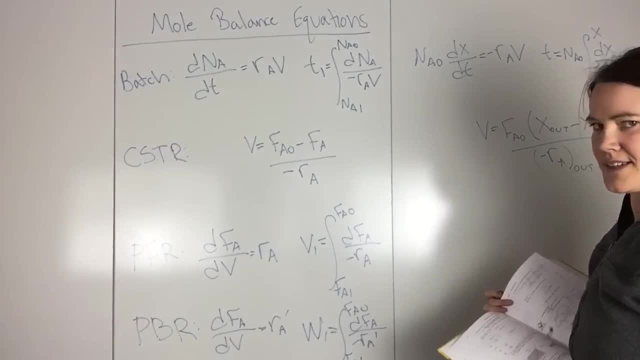 and you'll see that with these other two equations for the PFR and the PBR, because equations for the PFR and the PBR, because equations for the PFR and the PBR, because they could also have a reactor in, they could also have a reactor in. 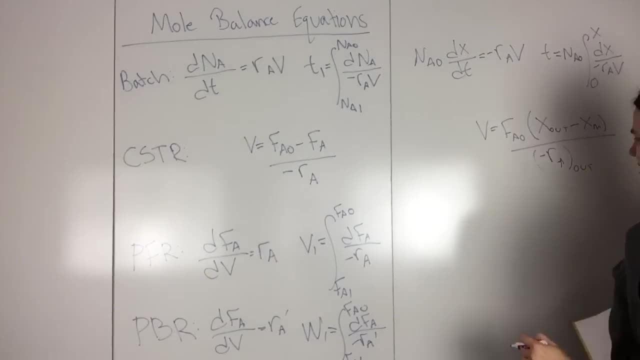 they could also have a reactor in series. so that's why this is the X out series. so that's why this is the X out series. so that's why this is the X out minus X in. so just remember: if so, I minus X in. so just remember, if so, I. 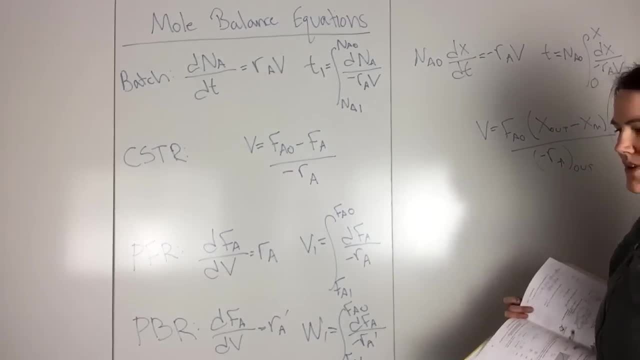 minus X in. so just remember, if so, I always start with this equation, and then always start with this equation, and then always start with this equation, and then, if I just have one reactor, and then I, if I just have one reactor, and then I, if I just have one reactor, and then I just say the X in is zero. so for the PFR, 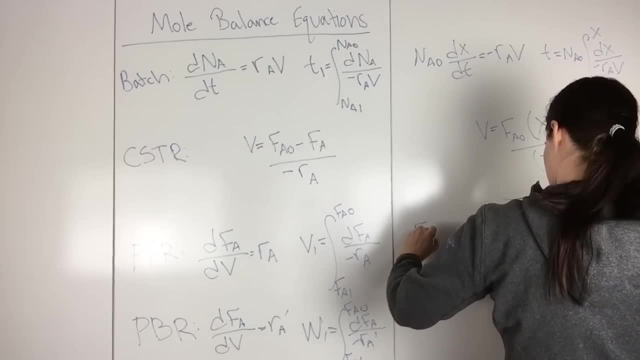 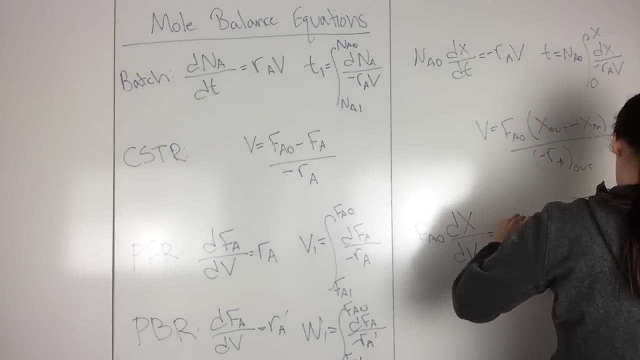 just say the X in is zero. so for the PFR, just say the X in is zero. so for the PFR, the design equation in differential form, the design equation in differential form. the design equation in differential form was FA, not DX. DB equals minus RA and 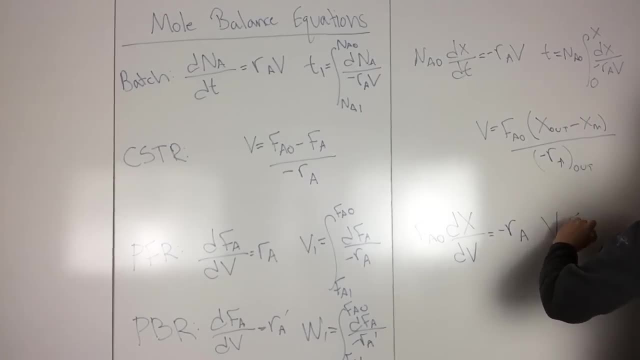 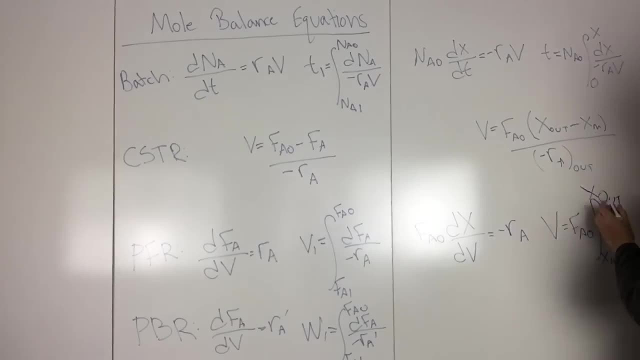 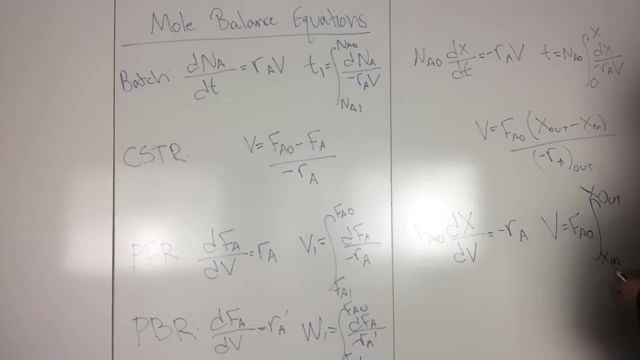 talking about. so this one: if you just have one PFR, then your X in is zero. but have one PFR, then your X in is zero. but have one PFR, then your X in is zero. but if you have some PFRs in series or you, 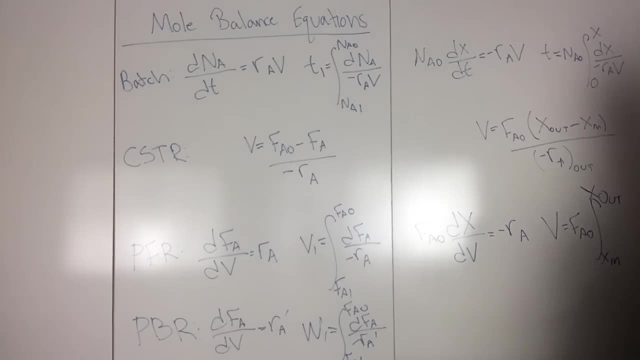 if you have some PFRs in series, or you, if you have some PFRs in series, or you have a CSTR and a PFR. so basically, if have a CSTR and a PFR, so basically, if have a CSTR and a PFR, so basically, if you have some flow reactors in series. 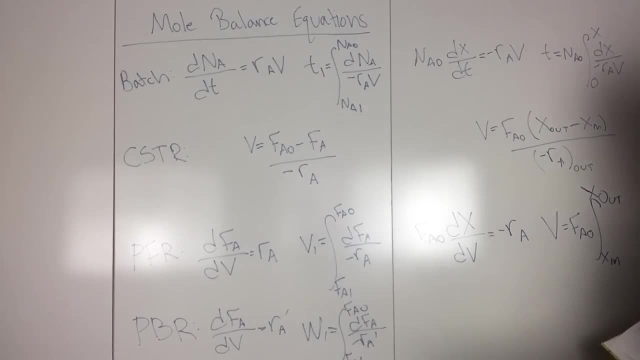 you have some flow reactors in series. you have some flow reactors in series. your X in is whatever the conversion was. your X in is whatever the conversion was. your X in is whatever the conversion was coming out of the reactor in front of coming out of the reactor in front of. 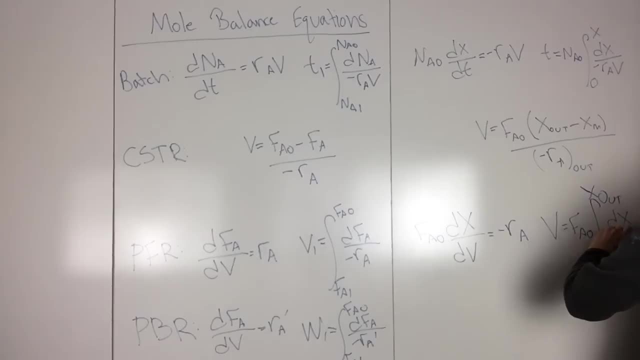 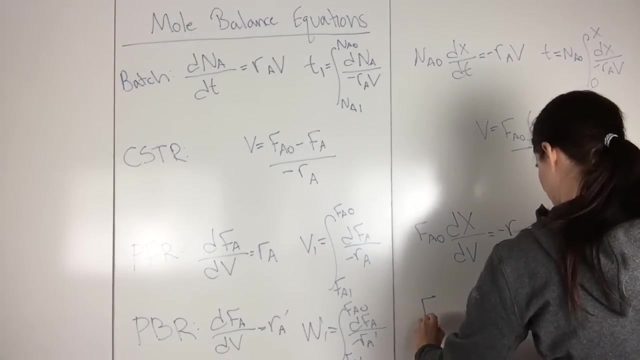 coming out of the reactor in front of it. so then this is D X over minus RA and it. so then this is D X over minus RA and it. so then this is D X over minus RA. and then for the PBR, the design equation is: then for the PBR, the design equation is: 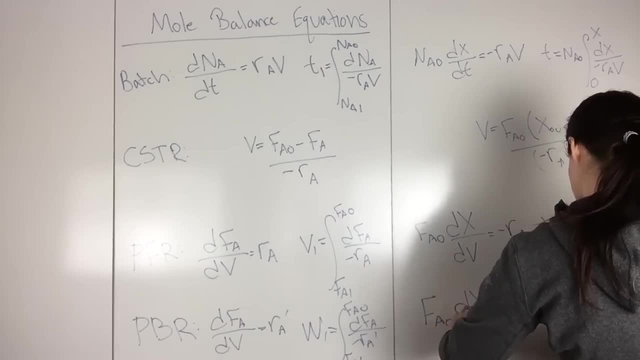 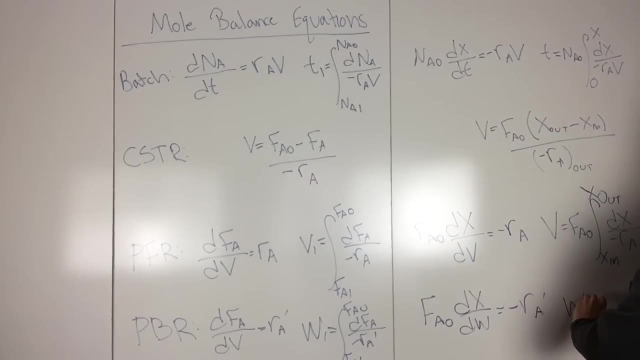 then for the PBR, the design equation is FA, not DX. DW equals minus RA prime in an FA, not DX. DW equals minus RA prime in an FA, not DX. DW equals minus RA prime in an integral form. it's FA, not X in integral form. it's FA, not X in. 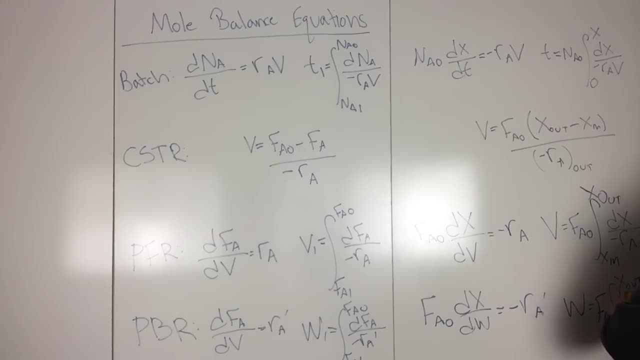 integral form. it's FA, not X in to X out DX over minus RA prime. so here's to X out DX over minus RA prime. so here's to X out DX over minus RA prime. so here's this again, the X into X out. so once this again the X into X out. so once. 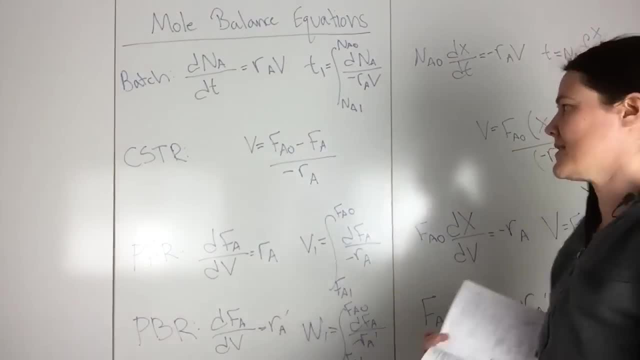 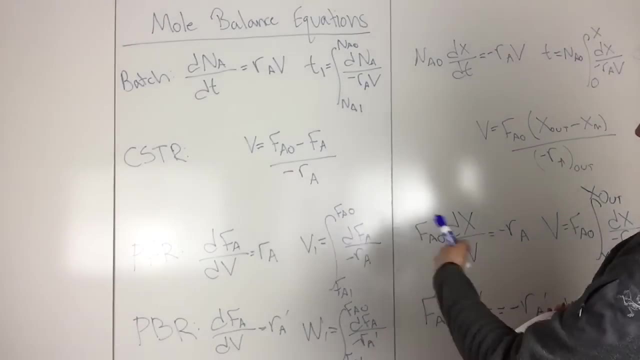 this again: the X into, X out. so once again these equations are in the chapter. again these equations are in the chapter. again these equations are in the chapter summary. so these are all chapter 1, these summary. so these are all chapter 1, these summary. so these are all chapter 1. these are chapter 2 and I would recommend: 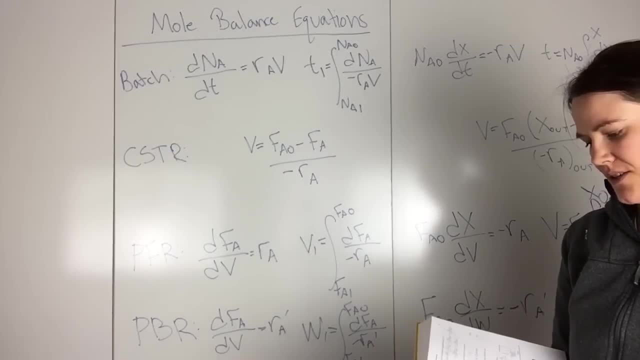 are chapter 2 and I would recommend are chapter 2 and I would recommend making a table of these in your notes. so making a table of these in your notes, so making a table of these in your notes, so then when you're doing, then when you're. 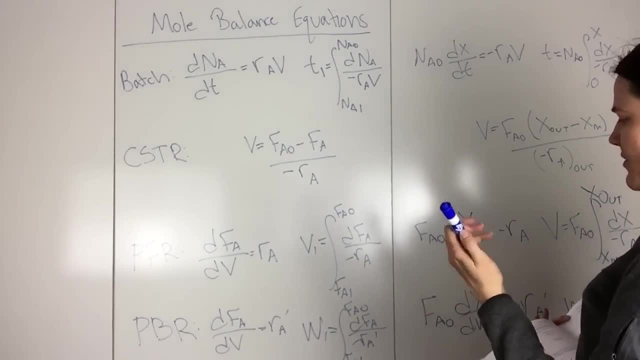 then when you're doing, then when you're, then when you're doing, then when you're doing assignments, so doing assignments, so doing assignments, so, or on an exam you can just reference, or on an exam you can just reference, or on an exam you can just reference. wherever you have this written down real. wherever you have this written down real, wherever you have this written down real quick, instead of flipping through the quick, instead of flipping through the quick, instead of flipping through the book and looking for these. 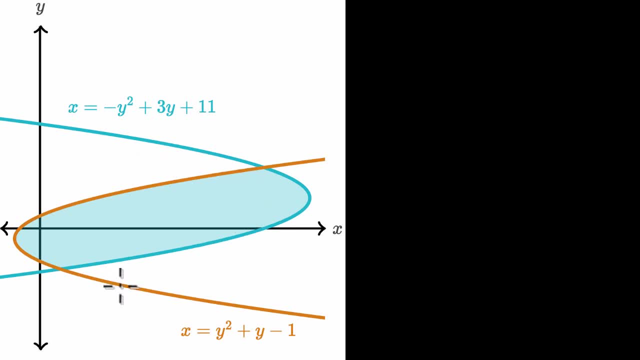 So I have two curves graphed here, and we're used to seeing things where y is a function of x, but here we have x as a function of y. In fact, we can write this top expression as being a function of y. 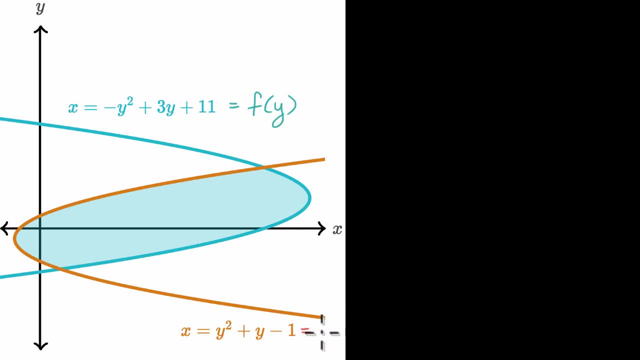 and this second one just to make it different. we could view this as g of y. Once again, it is a function of y, And what we're concerning ourselves with in this video is how do we find this area in this light blue color?